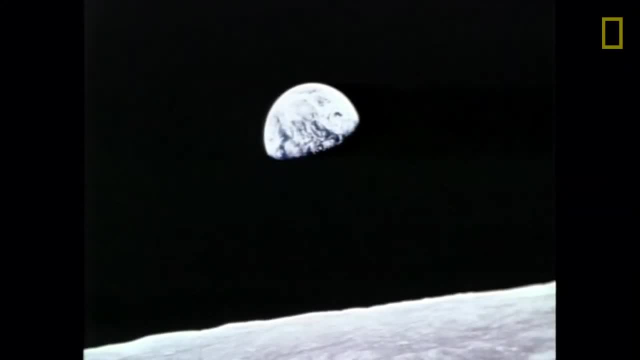 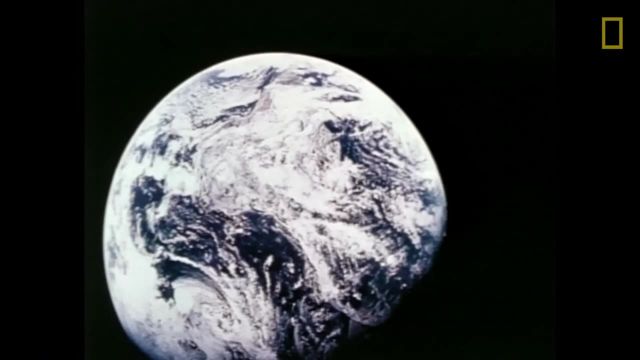 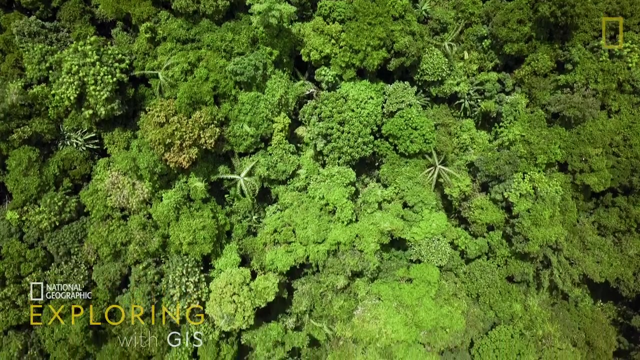 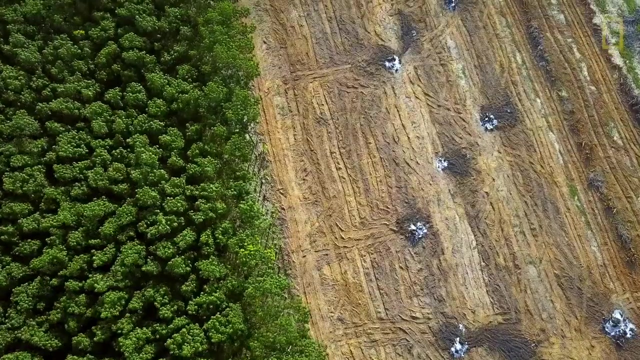 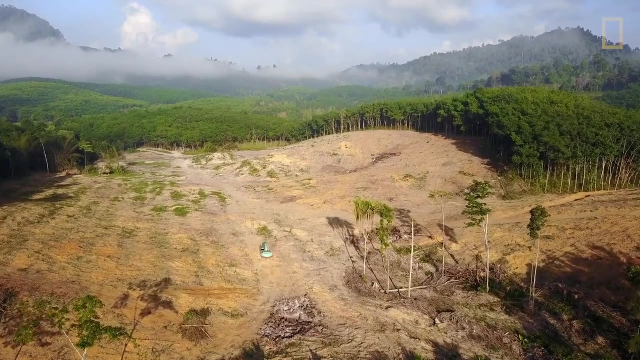 Oh, I remember those first pictures of the little blue and green planet from outer space. It was almost science fiction, almost I could hardly believe it, Seeing for the first time the extent of deforestation, The extent of how we, the most intellectual species, are destroying our planet. 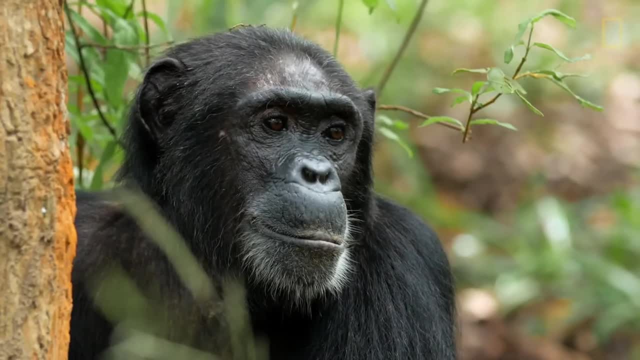 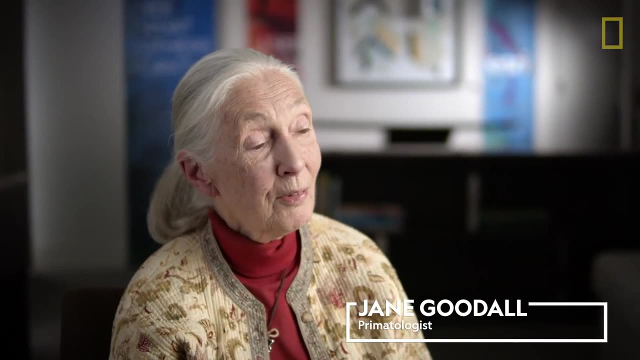 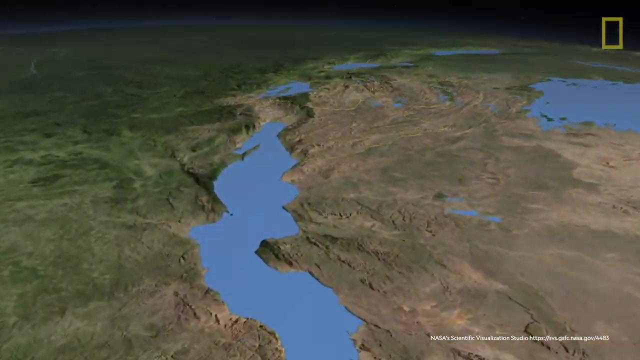 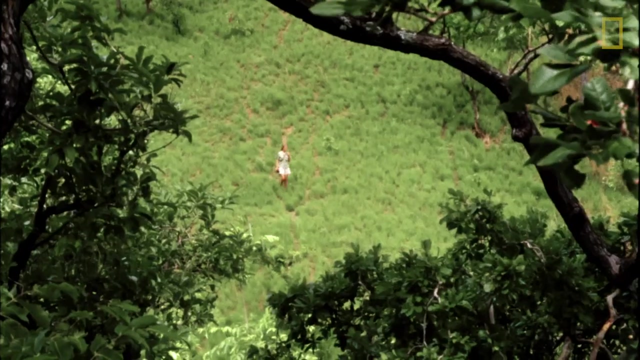 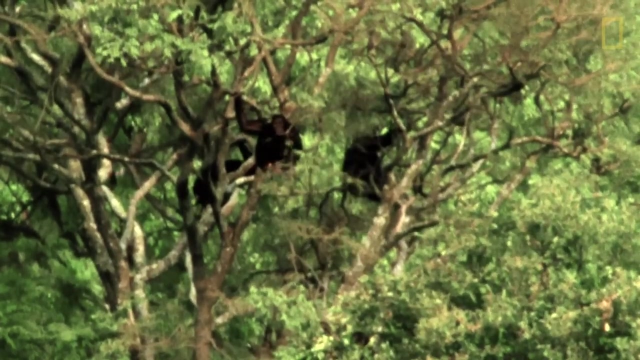 As ecosystems are destroyed, plant species, animal species will disappear. These are shocking things, but it should wake us up. We should be very, very alert now. Gombi is the smallest national park in Tanzania. When I began in 1960, Gombi was part of the equatorial forest belt that went all across. 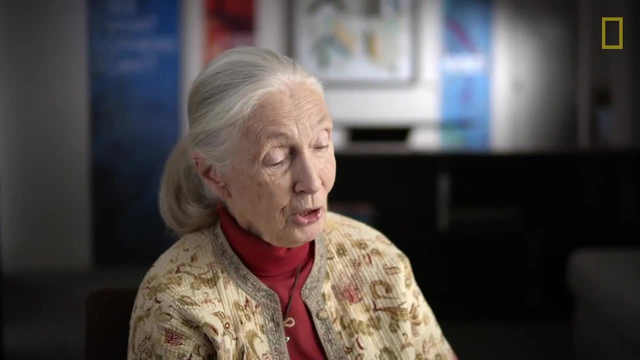 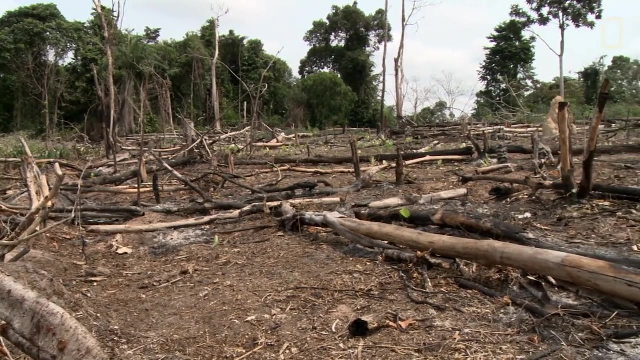 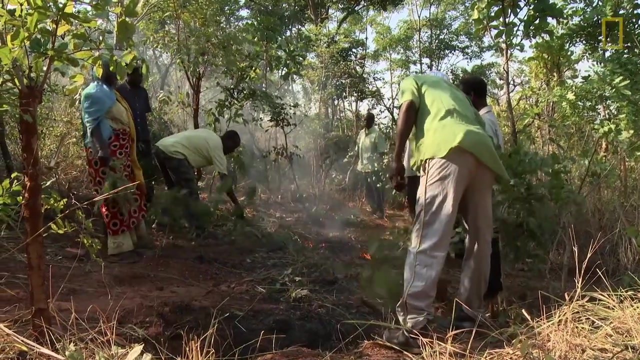 to West Africa By 1990, it was a tiny island of forest surrounded by completely bare hills. That's when it actually hit me. if we don't do something to help the people find ways of living that don't destroy the environment, we can't even try to save the chimpanzees. 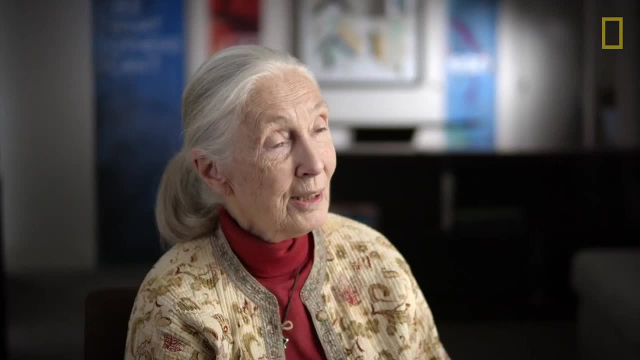 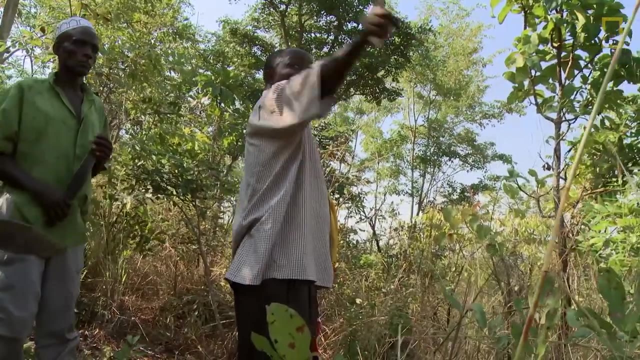 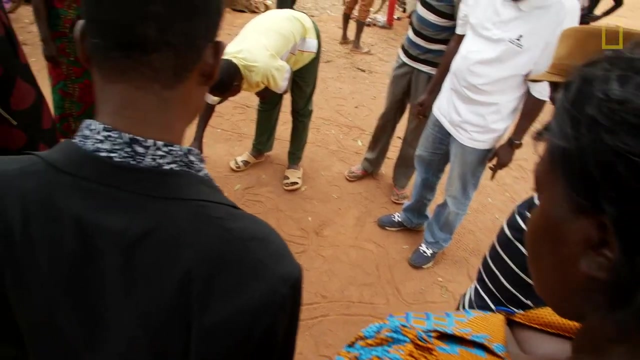 It was in 1994 that the Jüngerl Institute began its program. This idea of working with the people was sort of new. I mean others were handing out bits of money and jobs and things. I mean it was a new thing. 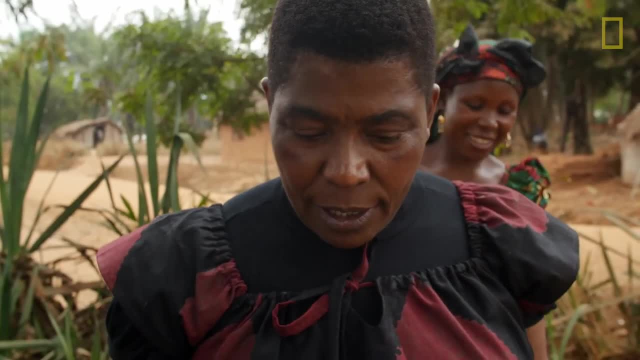 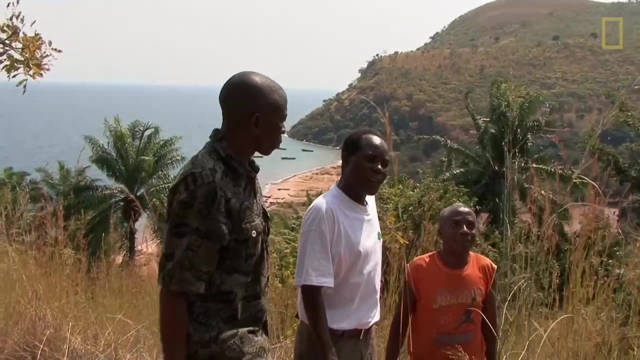 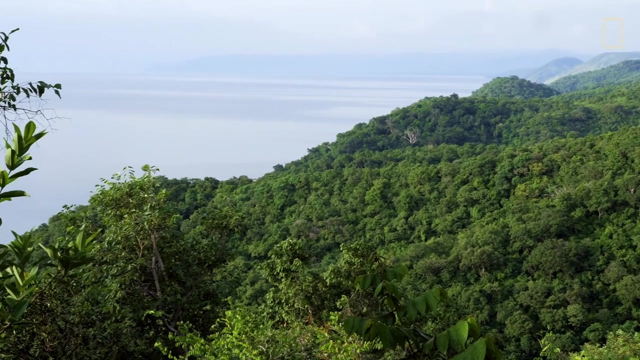 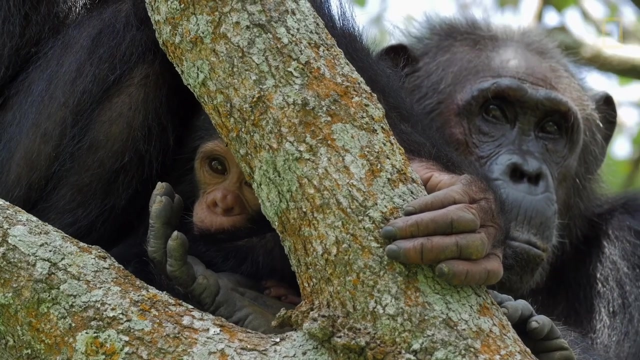 But this was working with the people. The trust that we built up is a very gradual process. Once the villagers had come to trust us, they began to understand that preserving the forest, the environment, was just as important for their own future as for preserving wildlife. 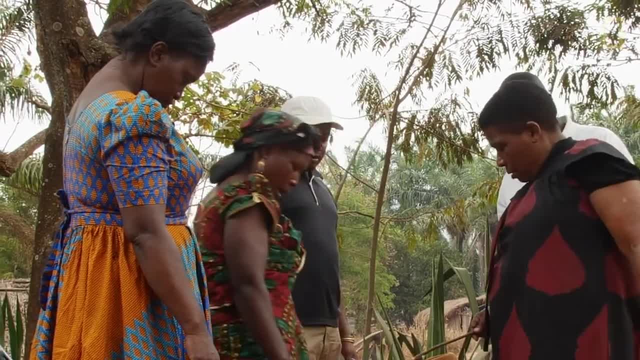 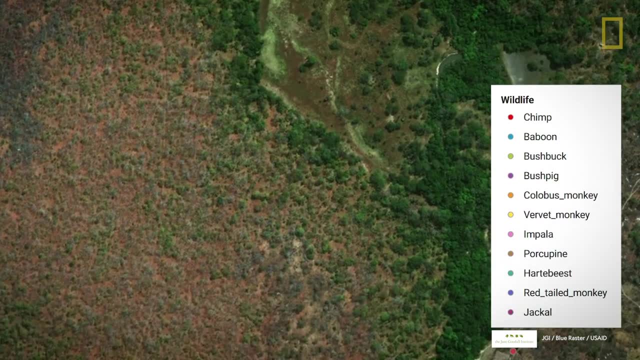 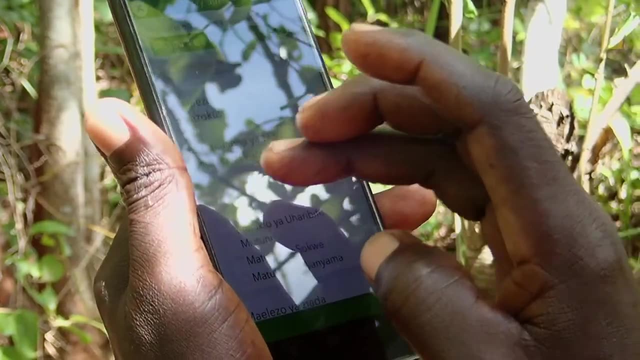 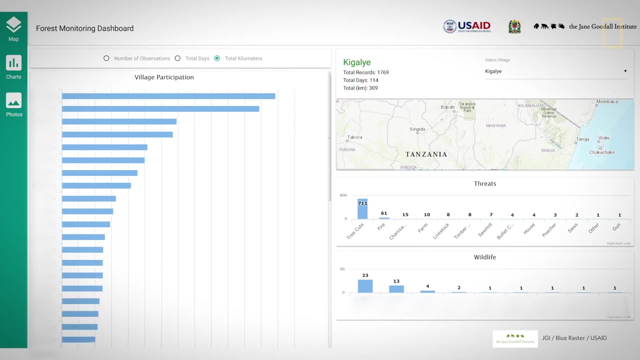 They got together all the data that they have decided is important. Whether it's an illegally cut tree or whether it's the sighting of a chimpanzee, The volunteer monitors all record the same things. They enter into their smartphone all the data, plug in and upload it. 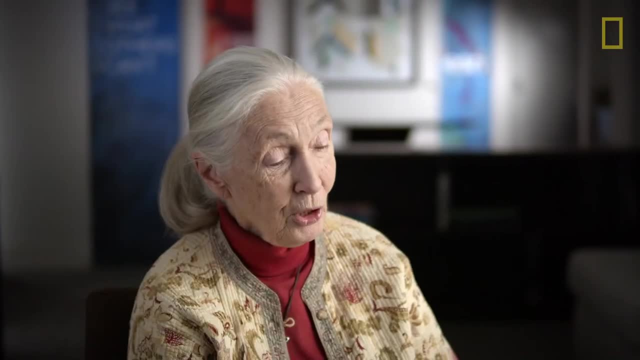 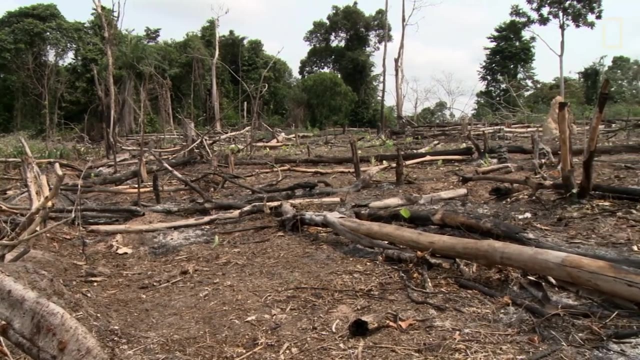 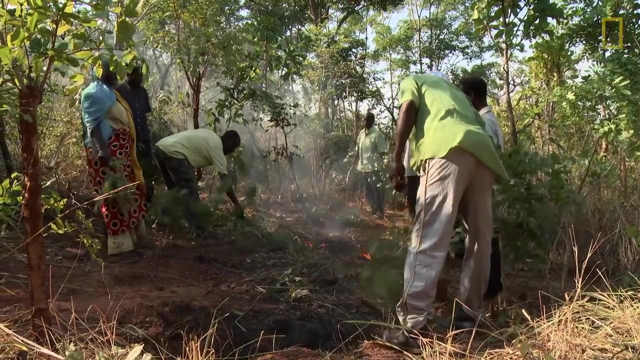 to West Africa By 1990, it was a tiny island of forest surrounded by completely bare hills. That's when it actually started. It actually hit me: if we don't do something to help the people find ways of living that don't destroy the environment, we can't even try to save the chimpanzees. It was in 1994 that the Jungerl Institute began its program. This idea of working with the people was sort of new. I mean, others were handing out bits of money and jobs and stuff, But this was working with the people. 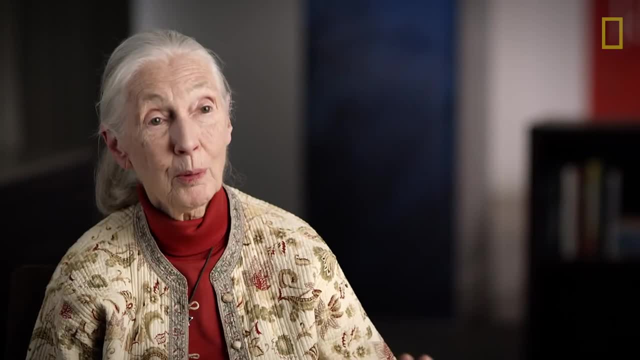 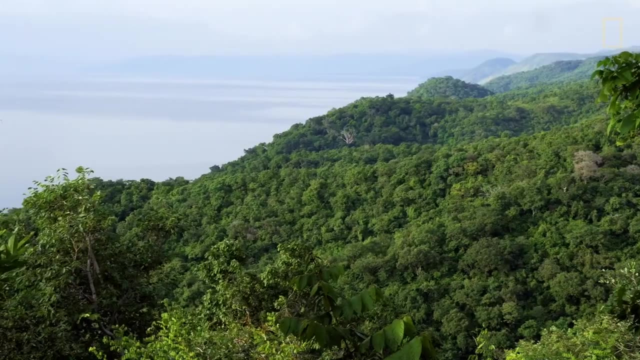 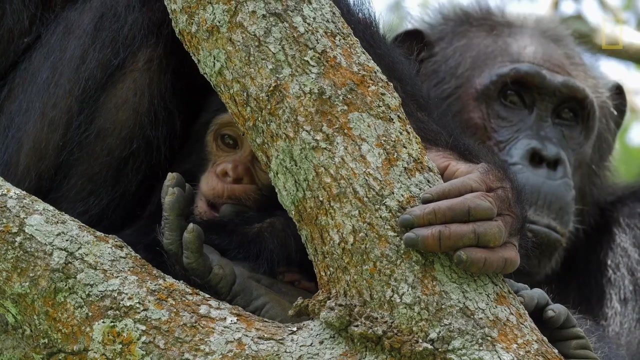 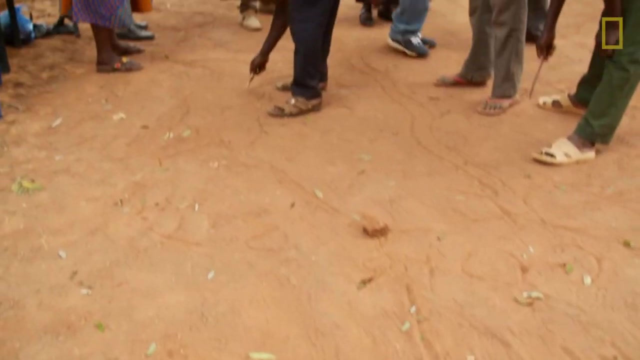 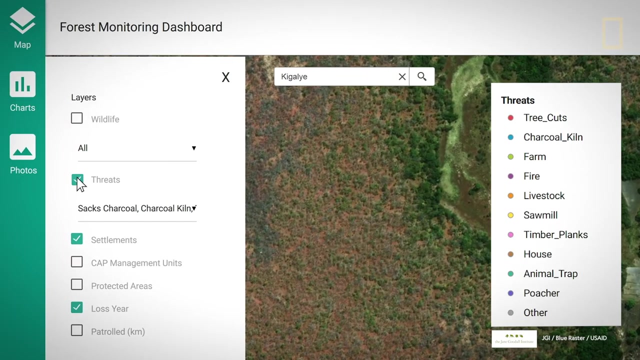 The trust that we built up is a very gradual process. Once the villagers had come to trust us, they began to understand that preserving the forest, the environment, was just as important for their own future as for preserving wildlife. They got together all the data that they have decided is important. 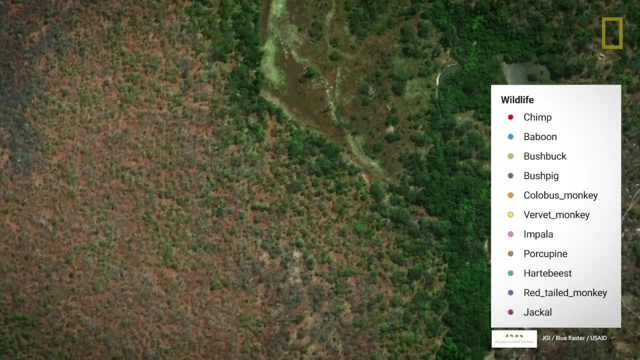 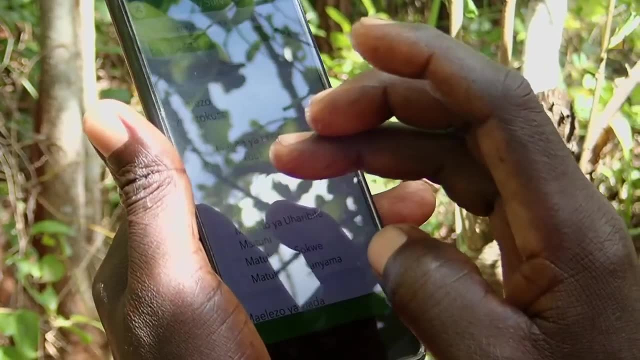 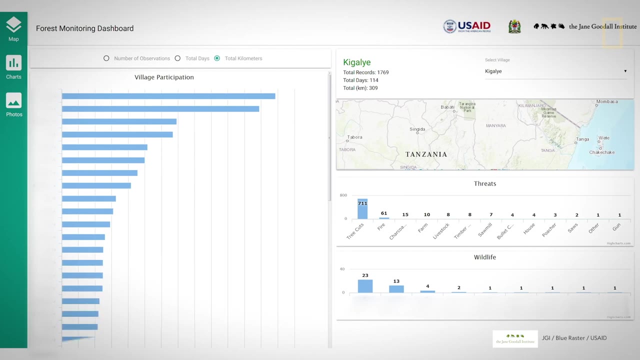 Whether it's an illegally cut tree or whether it's the sighting of a chimp nest, the volunteer monitors all record the same things. They enter into their smartphone all the data, plug in and upload it. GIS helps us see a picture of the environment. 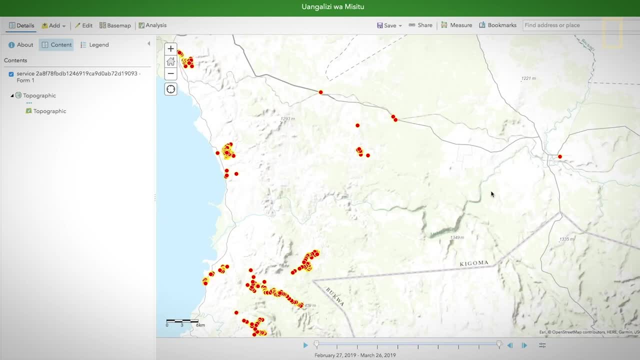 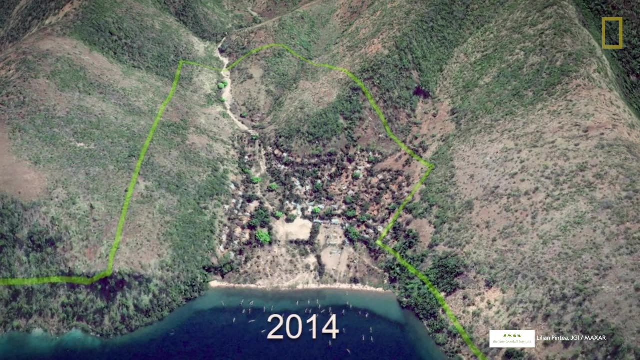 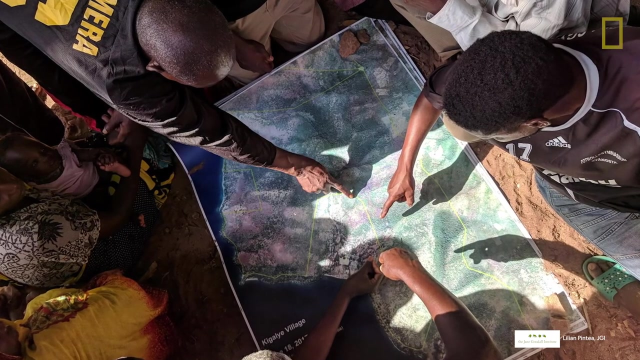 It's a very important part of our lives. It's a very important part of our lives. It's a very important part of our lives, The environment that we cannot see from down on the ground. That information becomes available to JGI, to the village leaders, as part of a picture. 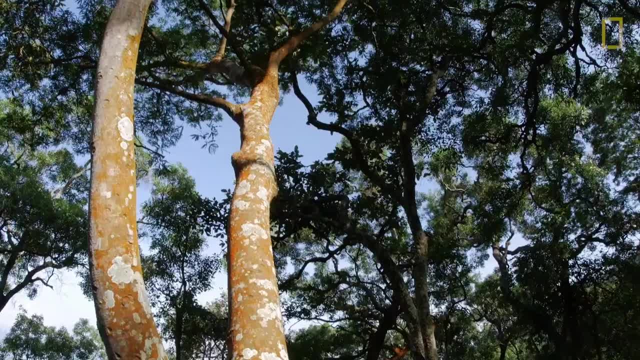 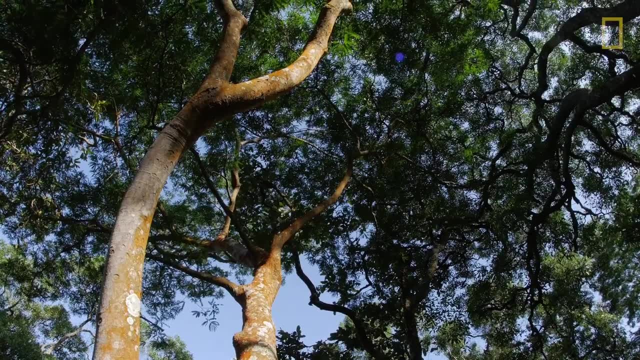 of what's going on around the globe. It's been shown in some forests where chimpanzees and other large animals have been hunted out. It's been shown in some forests where chimpanzees and other large animals have been hunted out. They don't have a voice. 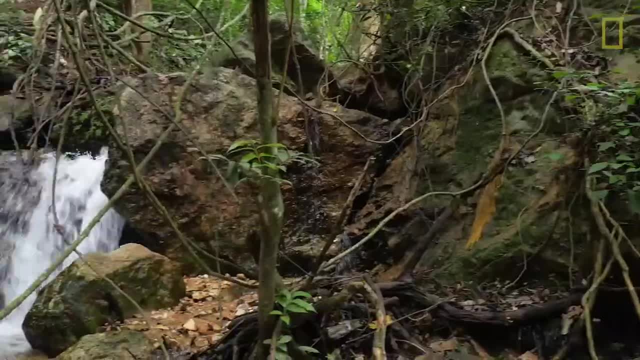 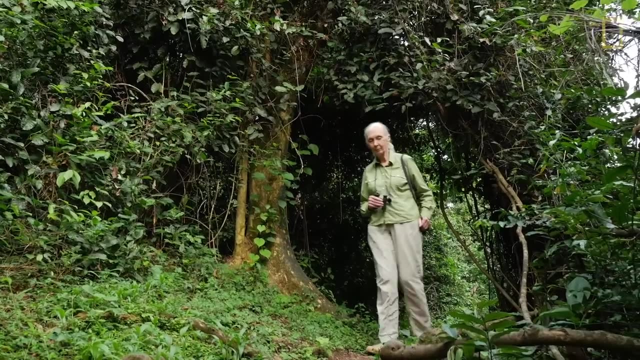 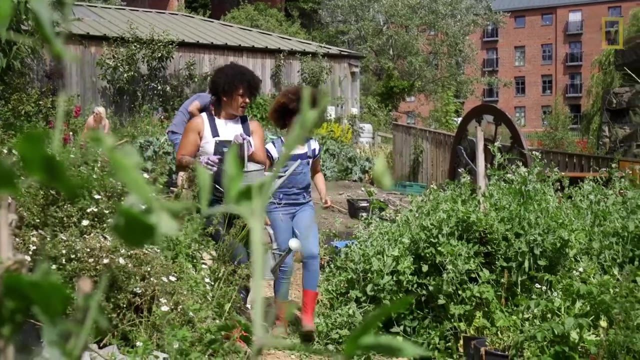 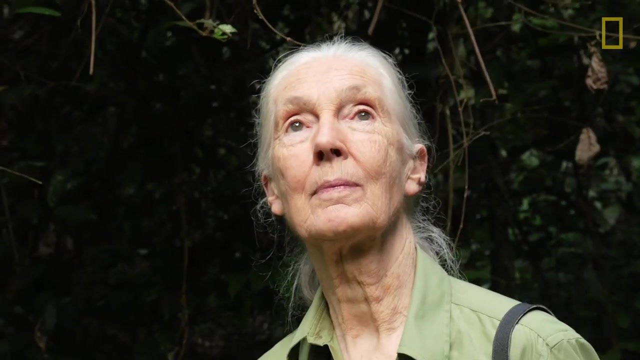 They don't know that the forest is not regenerating. So chimpanzees are a very, very important part of the forest ecosystem. Domitable human spirit, resilience of nature, the energy and commitment of youth, this incredible intellect, Those are my reasons for hope. 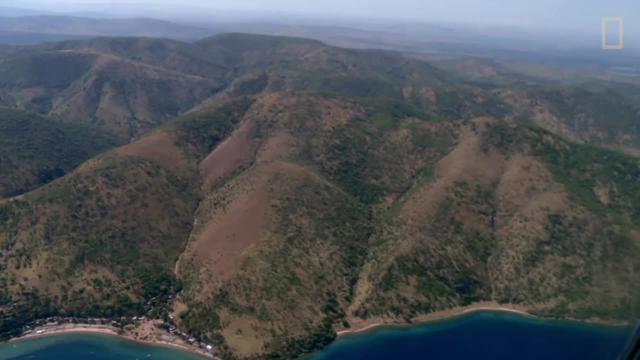 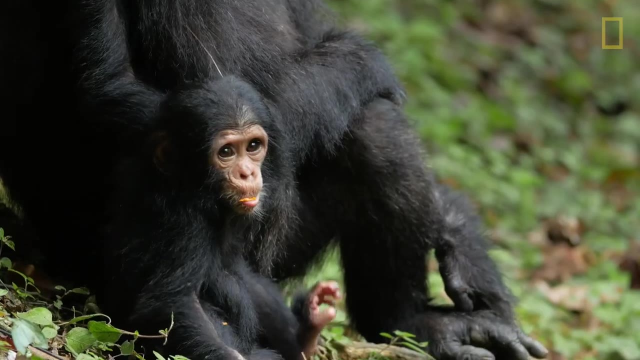 If we get together now, it's not too late, too late, We can solve the problems. We can, We must, We will.